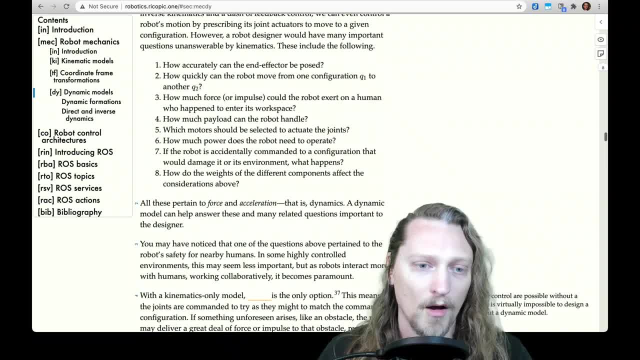 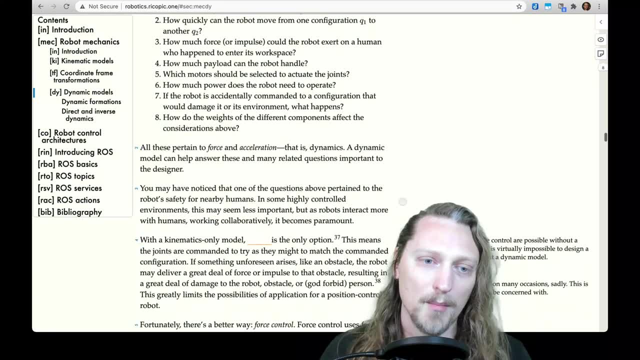 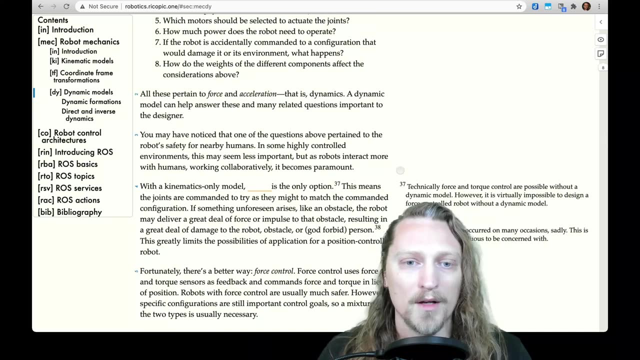 components affect the considerations above. All of these pertain to force and acceleration, That is, dynamics. A dynamic model can help answer these and many related questions important to the designer. You may have noticed that one of the questions above pertain to the 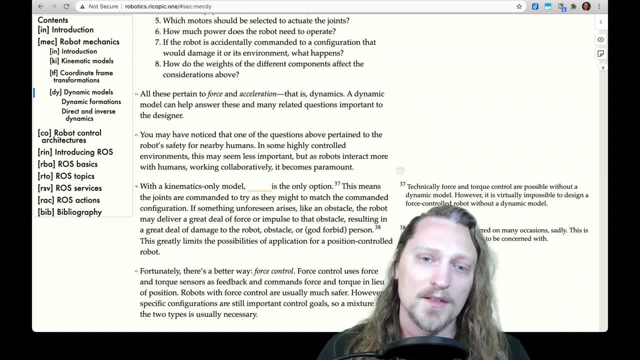 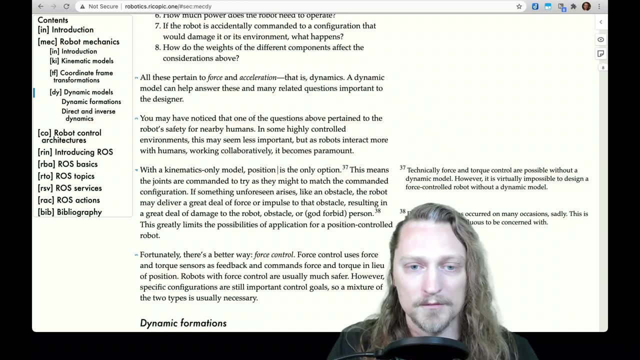 robot's safety for nearby humans. In some highly controlled environments this may seem less important, but as robots interact more with humans working collaboratively, it becomes paramount. With a kinematics-only model, position control is the only option. This means the joints are commanded to try as they might to match. 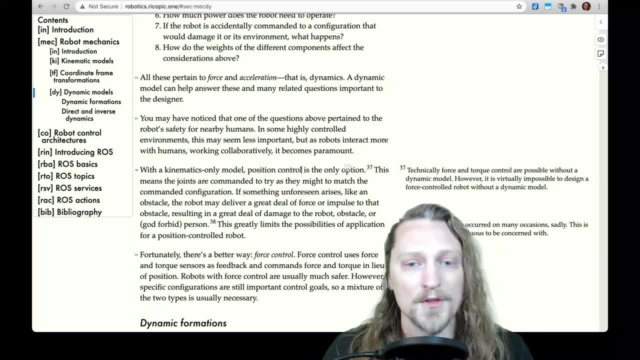 the commanded configuration. If something unforeseen arises, like an obstacle, the robot may deliver a great deal of force or impulse to that obstacle, resulting in a great deal of damage to the robot obstacle or- god forbid- a person. This greatly limits the possibilities of application for a position-controlled robot. 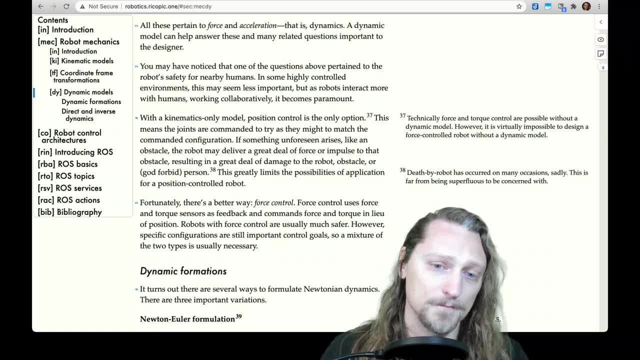 Fortunately, there is a better way: Force control. Force control uses force and torque sensors as feedback and commands. force and torque in lieu of position. Robots with force control are usually much safer. However, specific configurations are still important goals for control, so a mixture of the two types is usually necessary. 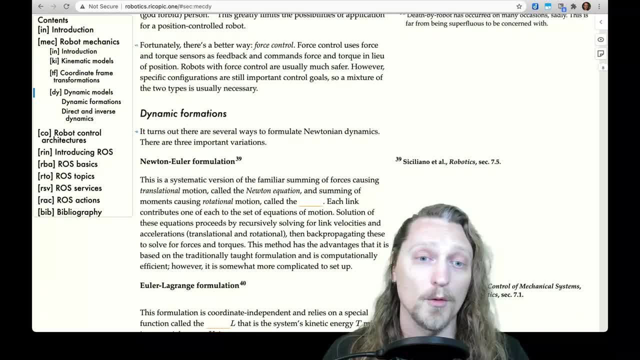 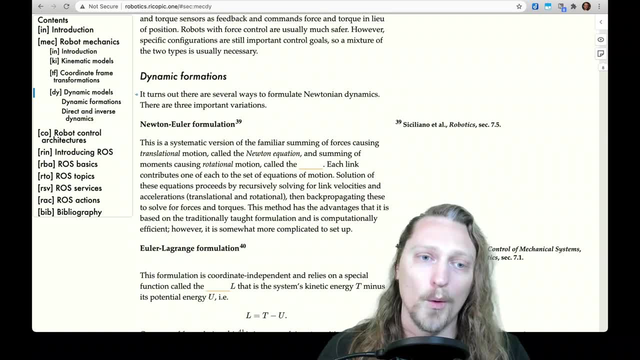 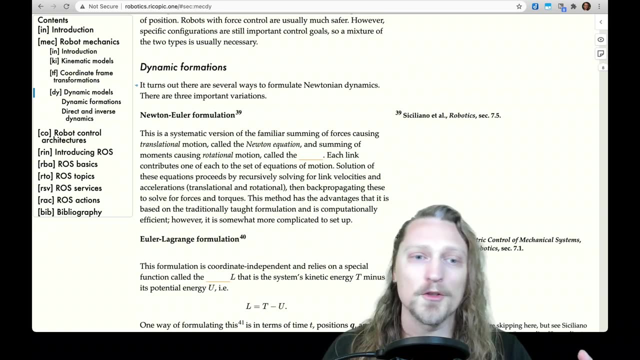 Dynamic formations. It turns out there are several ways to formulate Newtonian dynamics. There are three important variations: The Newton-Euler formulation- This is a systematic version of the familiar summing of forces causing translational motion, called the Newton equation, and summing of moments. 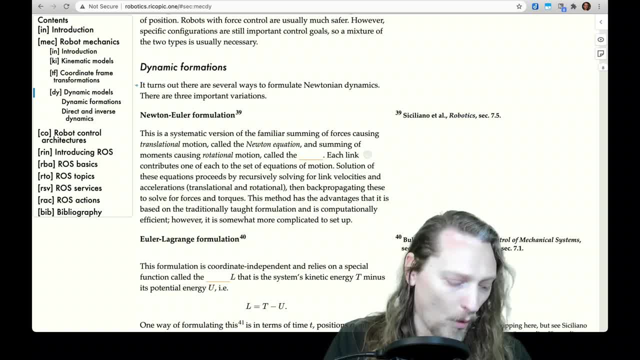 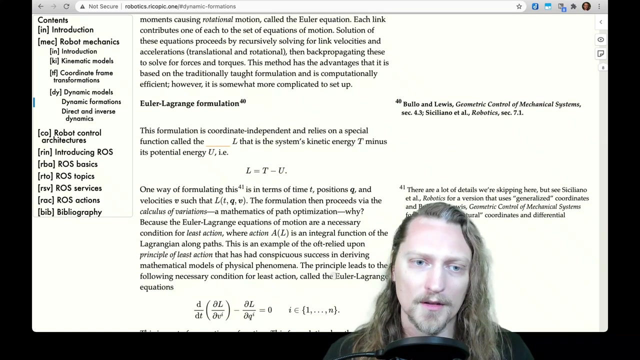 causing rotational motion, called the Euler equation. Each link contributes one of each, a bart of fy of time, requires the with it and is computationally efficient. However, it is somewhat more complicated to set up and doesn't extend as well The Euler-Lagrange formulation. This formulation is coordinate. 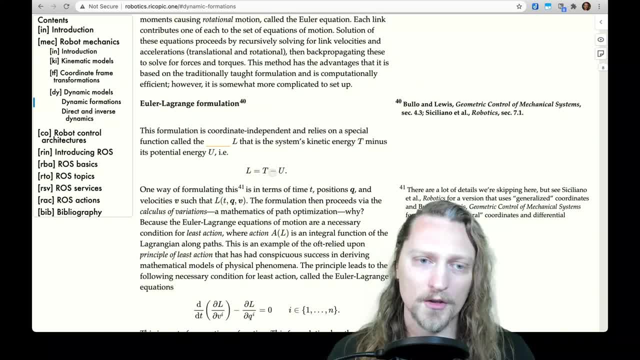 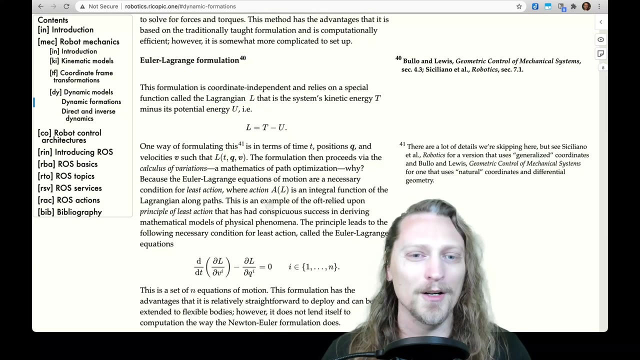 independent and relies on a special function called the Lagrangian L. typically denoted that is the system's kinetic energy, t minus its potential energy, u, ie t minus u. One way of formulating this, and there are many, is in terms of time t, positions q and velocities v, such that 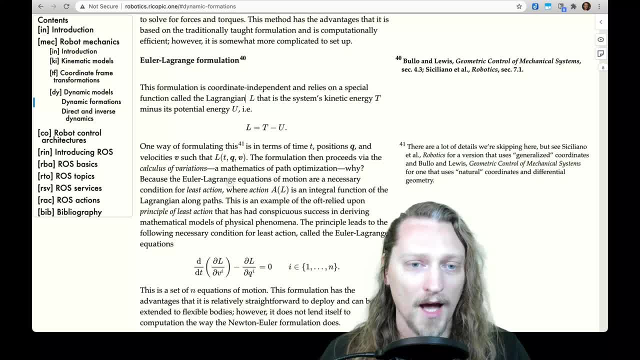 L. the Lagrangian is a function of time, position and velocity. The formulation then proceeds via the Euler-Lagrange formulation, The calculus of variations, A mathematics of path optimization. Why? Because the Euler-Lagrange equations of motion are a necessary condition for least action, where action a function of 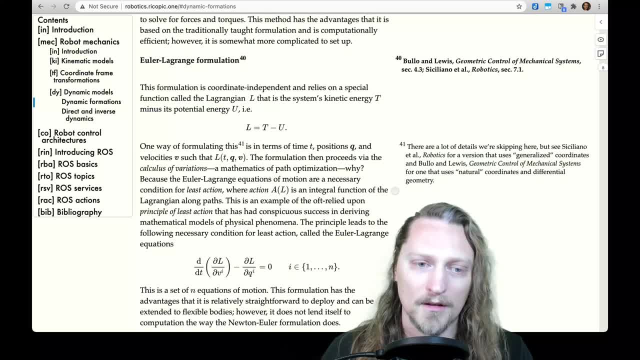 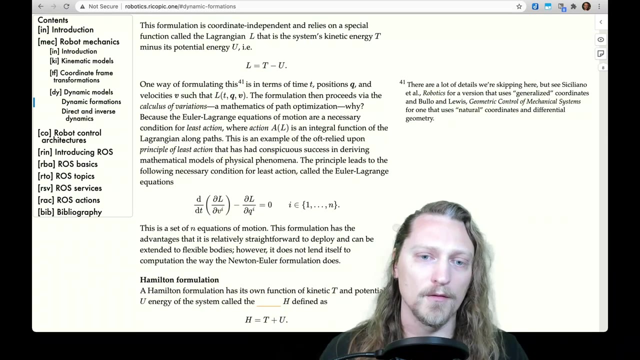 the Lagrangian is an integral function of the Lagrangian along different paths. This is an example of the oft-relied-upon principle of least action That has had conspicuous success in deriving mathematical models of physical phenomena. The principle leads to the following necessary condition for least action, called the Euler-Lagrange. 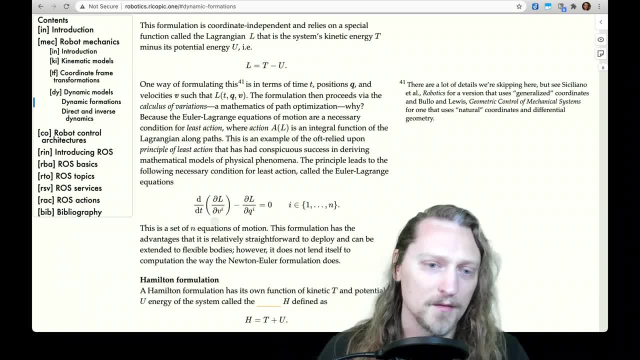 equations We have this time derivative of these partial derivatives of the Lagrangian with respect to the velocity coordinates, and this other term, the Lagrangian, is the neutral derivative or the partial derivative of the Lagrangian with respect to the spatial coordinates. 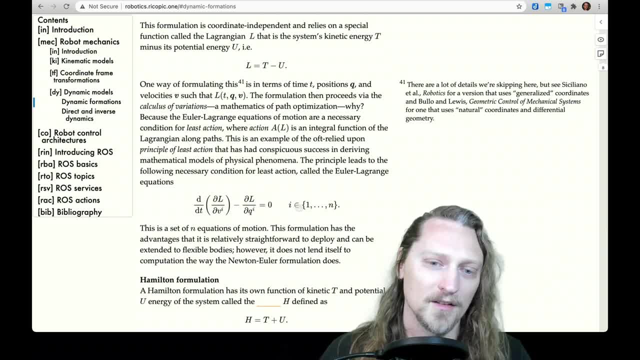 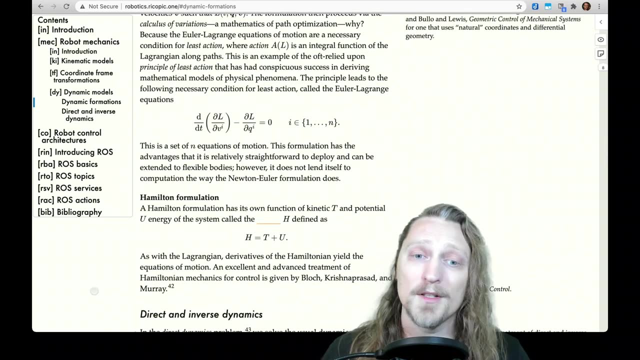 Now there are n equations, one for each coordinate I in this list of n indices. So this is a set of n equations of motion. This formulation has the advantages that it is relatively straightforward and can be extended to flexible bodies. However, it does not lend itself to computation in the way the Newton-Euler formulation does. 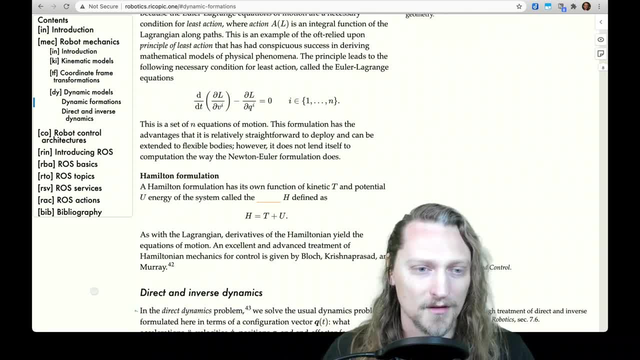 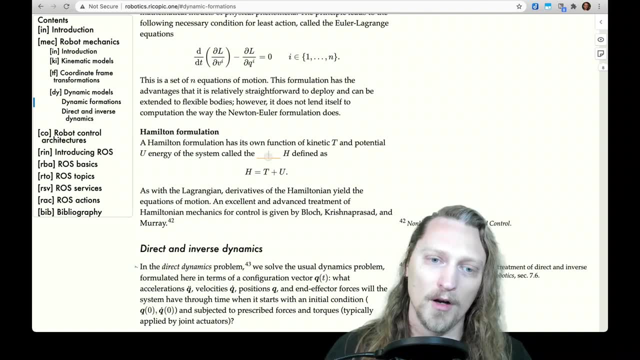 The Hamilton formulation, the third and final formulation. A Hamilton formulation has its own function of kinetic and potential energy of the system, called the Hamiltonian H, defined as T plus U, As with the Lagrangian derivatives of the Hamiltonian yield, the equations of motion. 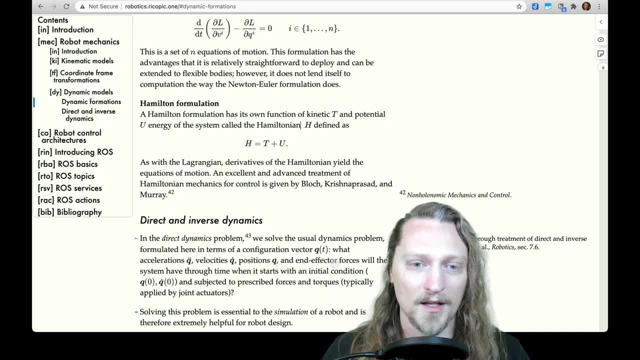 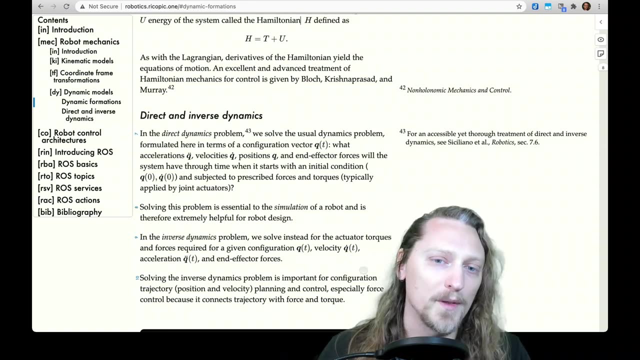 An excellent and advanced treatment of Hamiltonian mechanics for control is given by Bloch, Krishnaprasad and Murray. Direct and inverse dynamics. In the direct dynamics problem we solve the usual dynamics problem formulated here in terms of a configuration, vector q, a function of time. 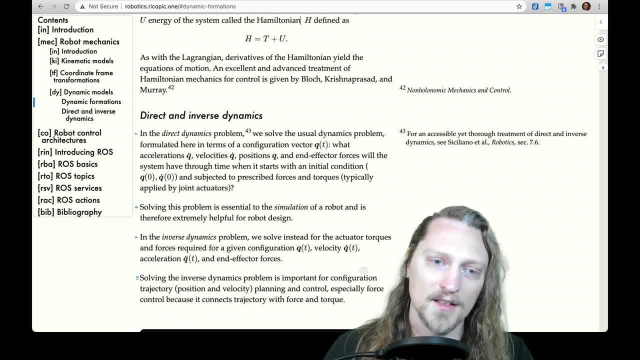 What accelerations q, double dot velocities, q, dot positions q and end effector forces will the system have through time when it starts with an initial condition and is subjected to prescribed forces and torques, Typically applied in the following order: 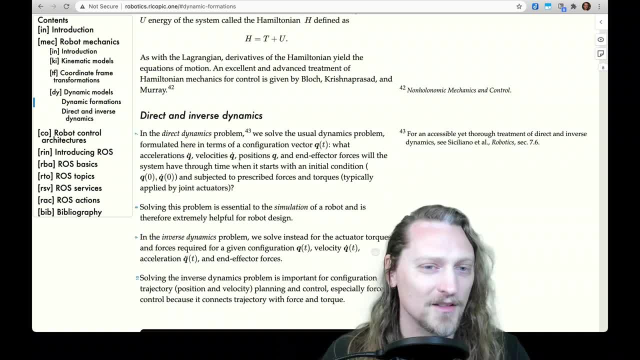 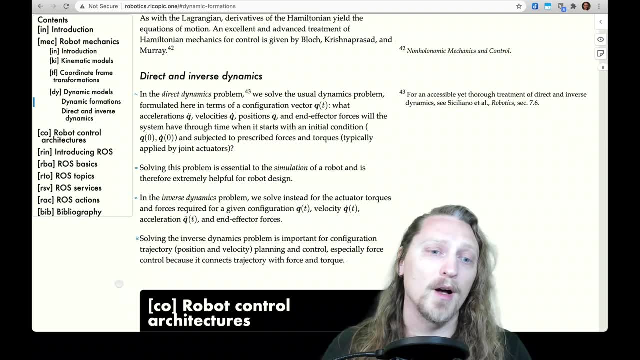 In the inverse dynamics problem we solve instead for the actuator, torques and forces required for a given configuration q of t, velocity q dot of t and acceleration q, double dot of t. Solving the inverse dynamics problem is important for configuration, trajectory, position and